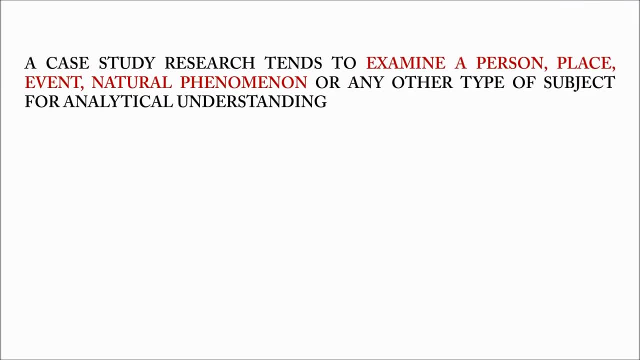 out Alright. so now a case study. research tends to examine a person, place, event, natural phenomena or any other type of subject for analytical understanding. So the main crux of the matter is analytical understanding of all these geographic facets that we are. 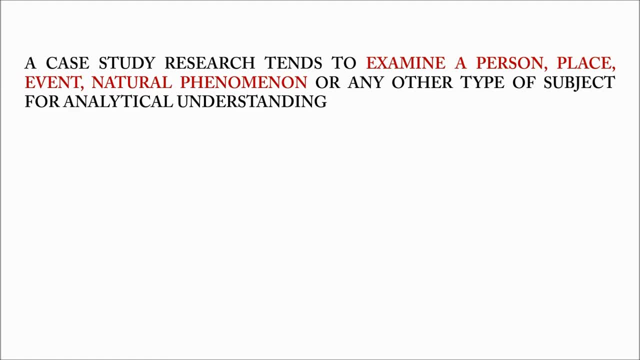 talking, people, places, interlinkages, natural phenomena. So these are the important aspects of a case study: research alright To bring out vital outcomes. it's also very much important to understand that it brings out vital, necessary items that are the important part of a broader framework of research. So 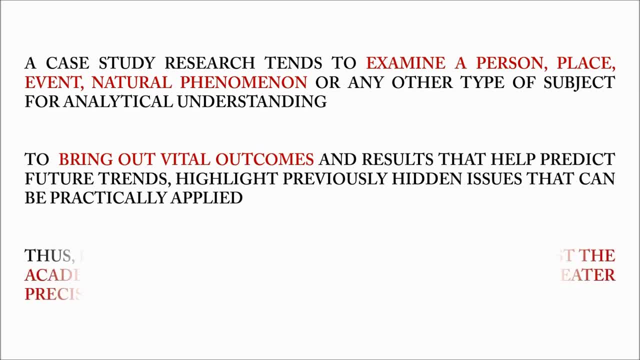 that is important because it's practically an applied format, isn't it? And it inculcates some means for understanding amongst the academic community. Okay, so now what I'm going to do. I'm going to give you a few examples of examples. You 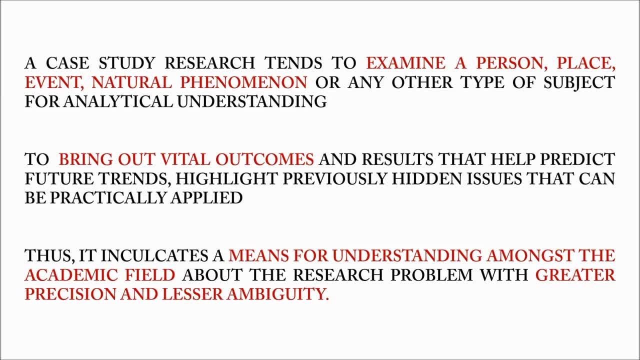 field. so that is also a contribution to academia. so the research problem with greater precision and lesser- you know, lesser- ambiguity. so precision has to be greater and ambiguity has to be minimized. so case study helps us to do these kind of exercises where we become more meaningful in 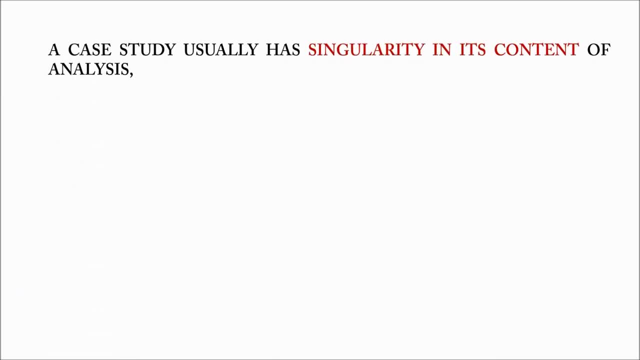 the academic field right. so a case study usually has singularity in its content. so case study is about very specific. very singularity is the common nature of the analysis in case study. but it may also be comparative analysis or comparative research or maybe interrelational research between two or more than two subject. matters that it can also be done in the case. 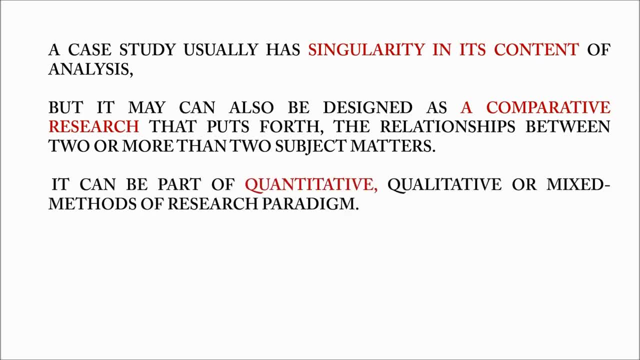 study part, so it can be part of quantitative as well as qualitative, or we can mix both the research methods. that is, quantitative and qualitative. often people tend to use mixed methods in geographical case study as well. all right, so the main aspect of a case study lies in its scientific credential. remember it has 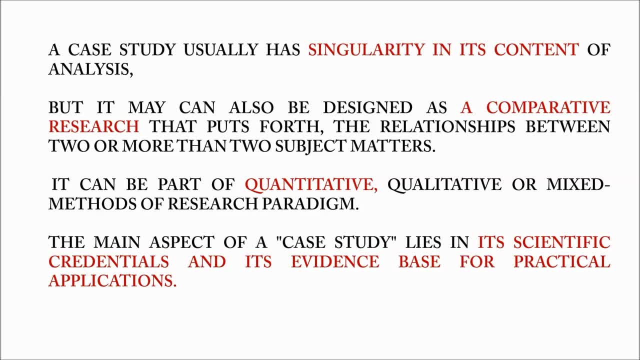 to be scientifically acclaimed, proven, and it's evidence-based for practical application. so the basic idea about a case study is: is it practical enough? that means, is it an evidence for the ground-based results? so it is important that we understand its practical applications. unless it is a case study, it cannot be a case study. it cannot be having a scientific credential, isn't it? so it 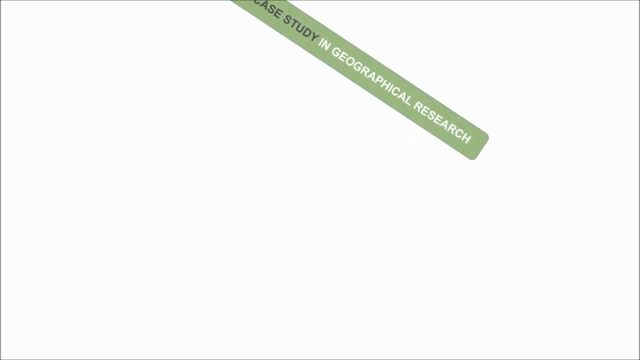 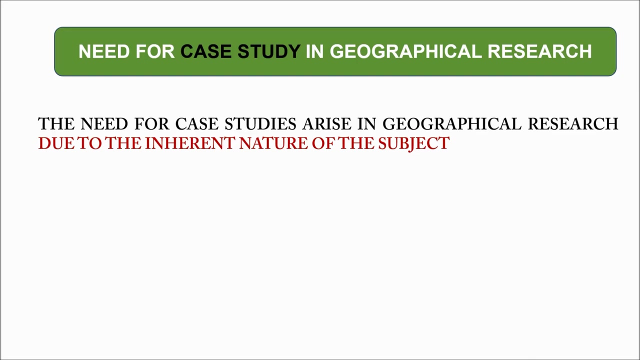 has to directly link to the. so now let's look at the need for case study in geographical research. why do we need case studies in geography? why is that subject matter related to case study? so let's look at that. the need for case studies arise in geographical research due to inherent nature of 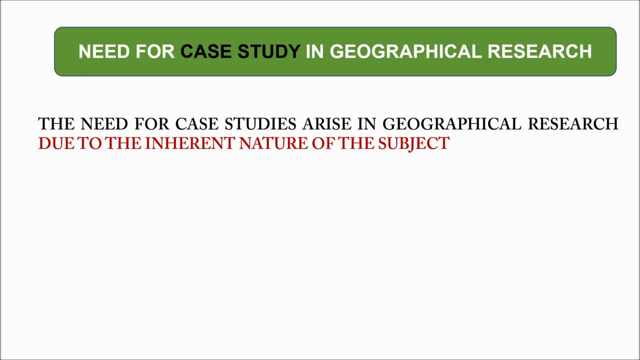 the subject itself. so, as we know, as we have already discussed about the definition, geography is all related to geography and geography is all related to geography and geography has multiple places and phenomena, and then interactions and several other components, isn't it so? case study deals with all. 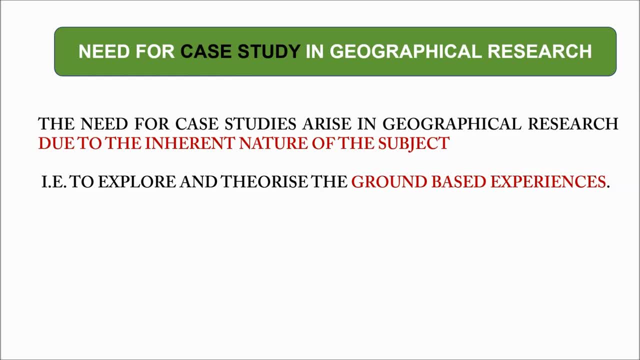 the same. so we explore and theorize. basis is ground. so what happens? we theorize from the ground experiences. that is what we have talked in the basic idea of fieldwork in geography. so making a case study is about backing up one's argument with examples from the real world. so if i'm making a 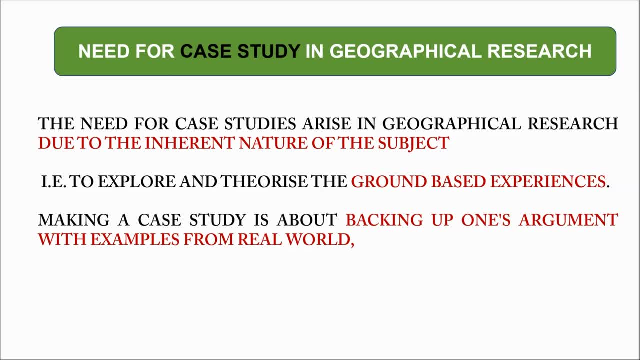 making about a real world situation through my case study. right so to show that one is aware and practically understands the real world situation. so what is happening on the ground? we have to prove it to make a case study. so unless we make a meaningful case study- which 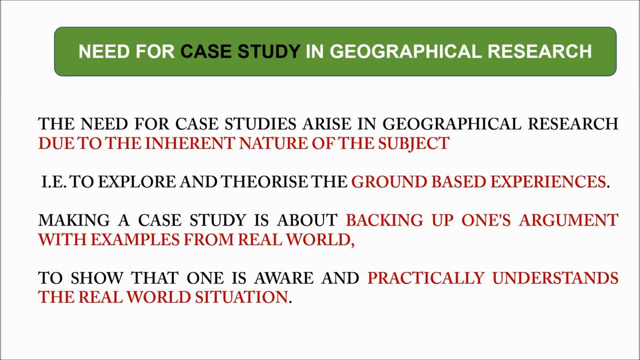 is scientifically valid and also it has rationals on the ground level and it has less of ambiguity, then it has a validity in the academic fraternity. so what happens? we do case studies in geographical research to bring out the practical understanding of the real world situation that we go to the 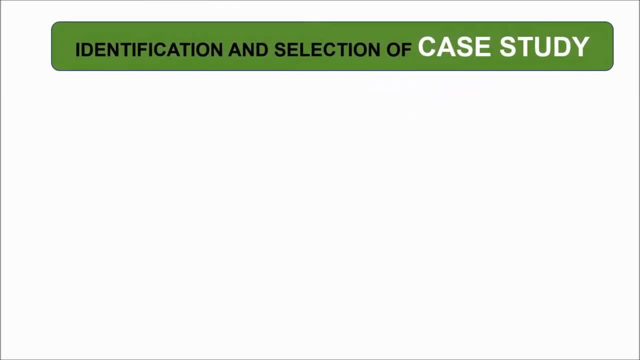 field right. so identification and selection of case study: it becomes very much important: how do we identify and how do we select a case study? what are the parameters for that? so let's look at that. identifying a case study to carry out research involves much more than just a research problem. so even if we have 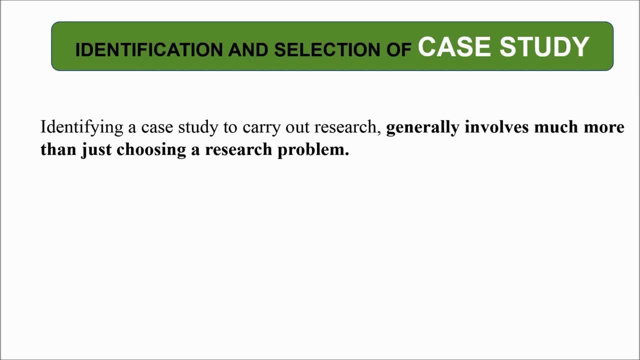 a research problem in hand. suppose i want to study a river pollution at some particular river. it's just a research problem, right? so it doesn't qualify for a case study unless it encompasses a contextualized situation on the ground. so we need to understand the context of the ground in. 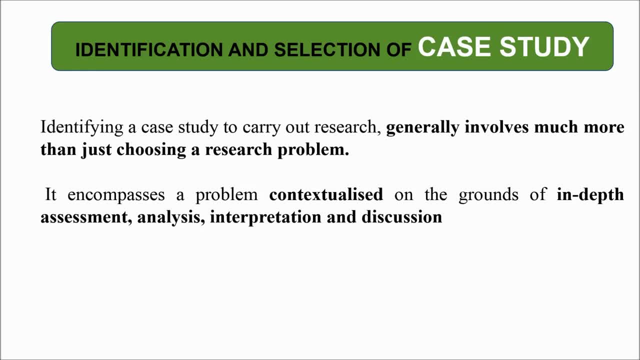 what context are we talking of? suppose a river pollution or a bond pollution or lake pollution. is it humanized? is it just in a natural state? what is happening there? so the context becomes really important and in-depth assessment, analysis, interpretation and discussion on the grounds are the important parameters. so that often results in specific recommendations for practical action on 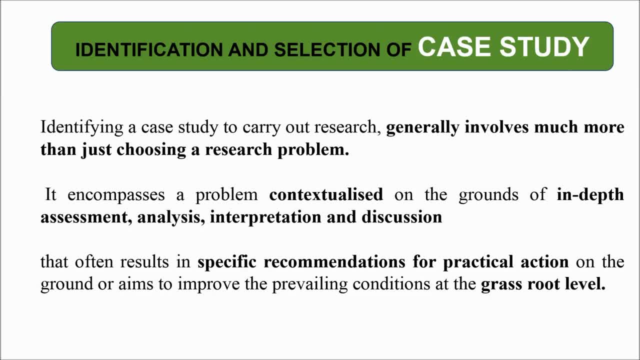 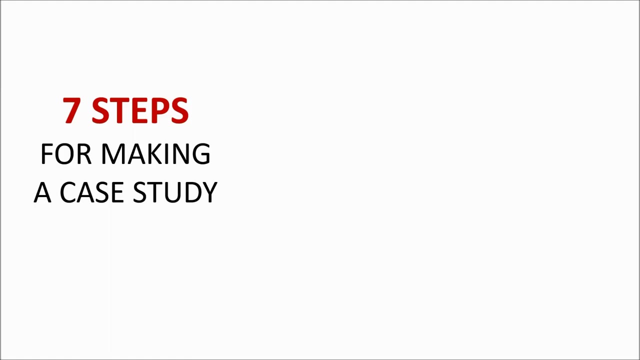 the grassroot level. so what happens here is, when we identify and select a case study, it must have a specific contextual, practical action on the ground, on the grassroot level. that is the whole idea about doing a case study in geographical research. isn't it now the seven steps for making a case study? now remember these seven easy steps to make a case. 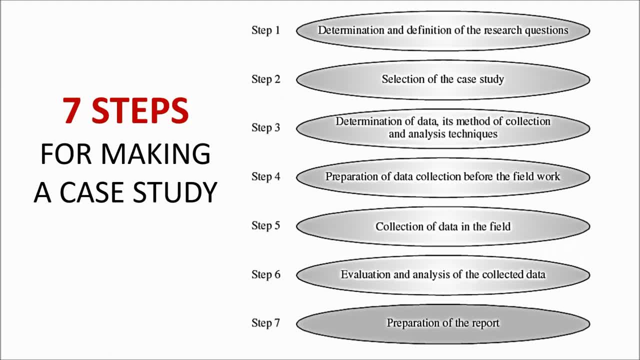 study that we are going to discuss. so let's see what is that. these are the seven steps. first is determination and definition of research questions. the first idea is that we must understand what are our pre-questions that we are going to ask. so what are we searching answers? 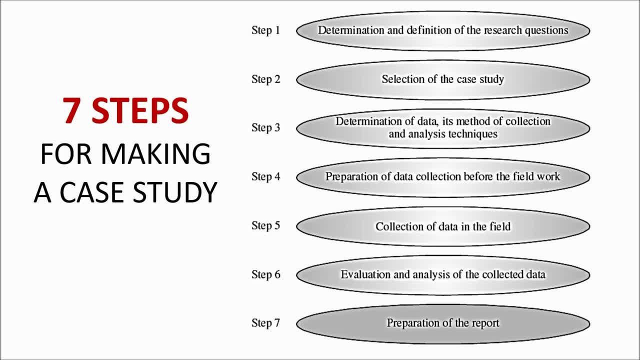 then selection of the case study, as we have already talked. so case study selection becomes really important. and then the determination of data, its method of collection and analysis. so that is the research methodology, part right, the database, and the research methodology becomes very much important. so, preparation of data collection before the field work, collection of 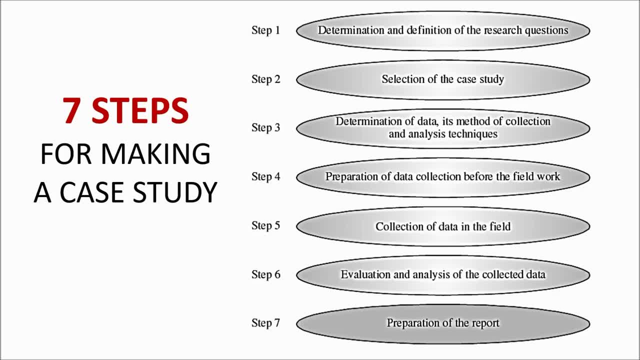 data in the field, evaluation and analysis of the collected data and preparation of the report. so these are the seven easy steps to conduct to make a case study, okay. so if you want to revise it, remember first determine the research questions, then make a selection of case study, then 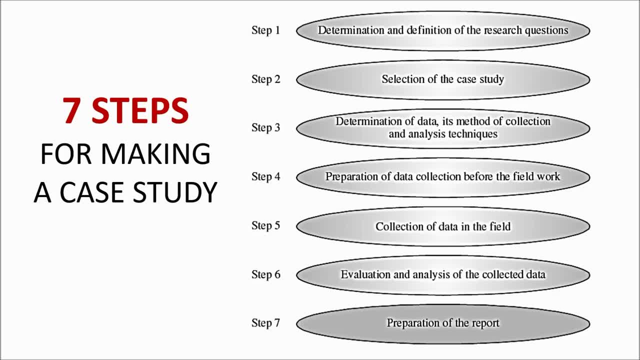 see what is the database going to be, what are the methods of collection going to be and how are you going to analyze those data. isn't it then prepare a data collection method for the field work? so what are the methods in the field work that we are going to use for the 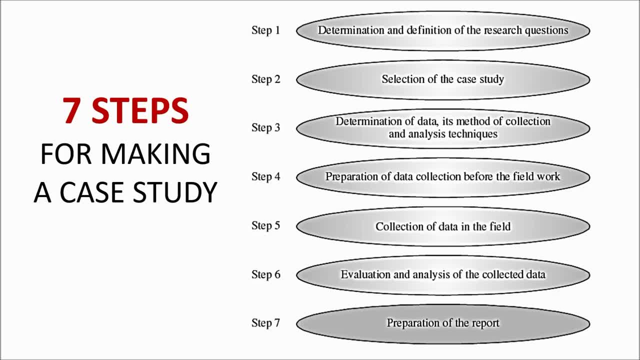 collection of data. how are we going to collect the data and collection of data finally, in the field. so first the planning stage till step four and then collection of the data in the field. then step six is about evaluation and analysis. this is very much important because it holds the 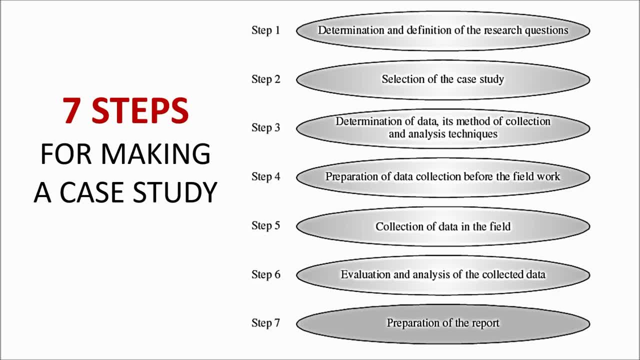 key to the outcomes that we are taking data from the ground. and then, finally, preparation of a report in the last stage. so these are the easy seven steps to understand how to make a case study. so if you want to make a case study, just remember these seven steps and plan each. 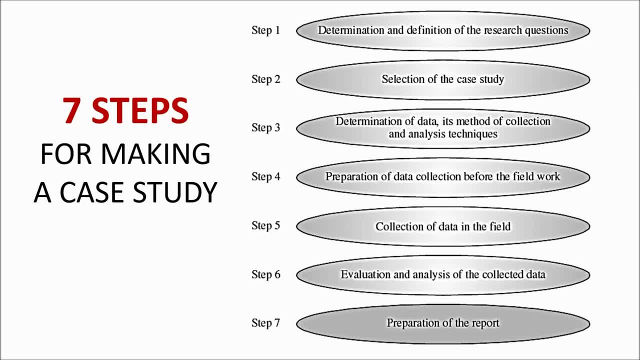 step very carefully and judiciously with time management and also with money management, because every research would take some amount of cost. so time and cost are two important things a researcher must take into consideration while planning for a case study. all right, so go ahead. now i'll tell. 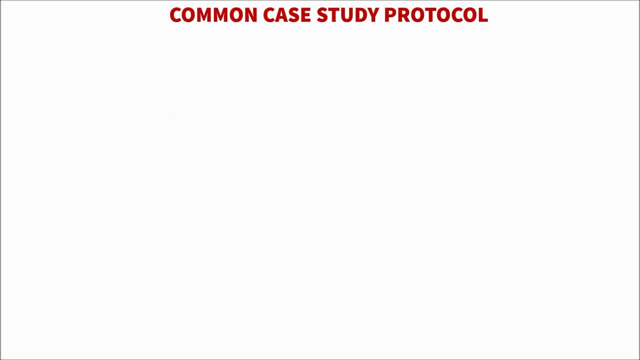 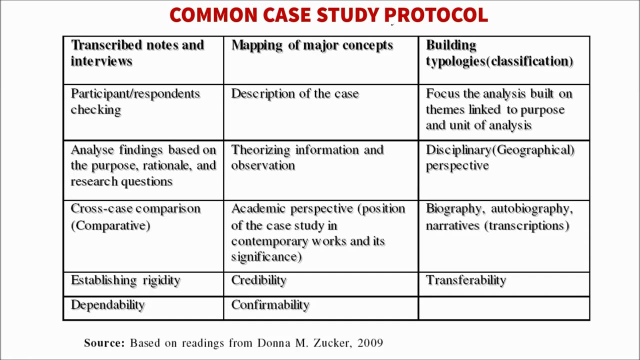 you about some common case study protocol that should be remembered, should be taken into consideration while making a case study. so look at these few of them. i'll just read out: this is important: that you must transcribe notes and interviews. so when we are taking interviews from people, we must write it into academic paper in academic format. then checking into 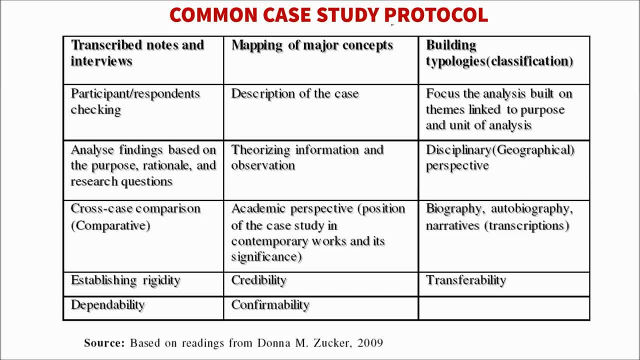 the findings based on purpose, rational questions, cross case comparisons, happening credibility, transferability, disciplinary perspective, theorizing information from the field. right cases are important. so largely these, all these factors that we are talking here is trying to build the validity, trying to make it more practical to the ground based situation. so these are the 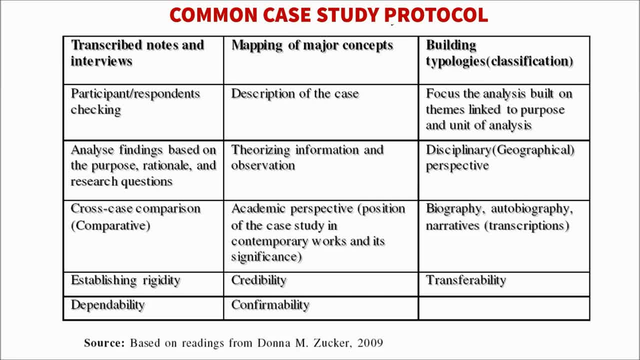 case study protocols that we must understand, must follow. that is my case study based on this protocol. are. am i following it? so you need to question yourself, depending upon this common case study protocol, what is the case study protocol and what is the case study protocol? so these are the important case study protocols that one must follow in order to validate one's 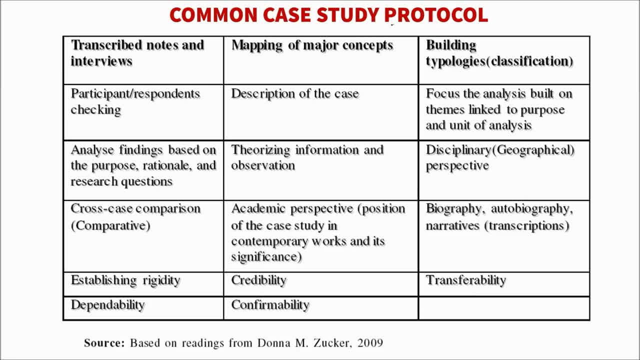 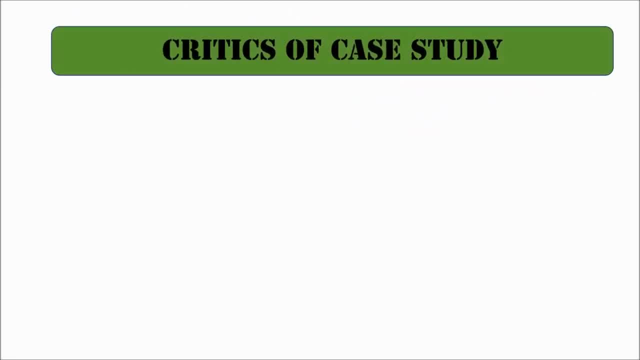 case. all right, so these are the list, then now let's look at the critics of case study. many people feel that case study is not that important. so what are their arguments? the critics of case study research normally tend to be critical of case studies, and they tend to be critical of case. 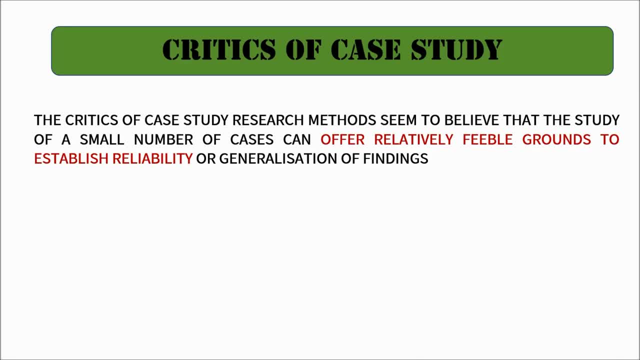 studies, and they tend to tell us that- offer relatively feeble grounds for establishment of reality because they are very small numbered, they are very contextual, so generalization is not possible on a case study basis. so this is the first critique: that case study is very specific. it cannot be generalized to overall findings, isn't it? so that is the first critique. then many 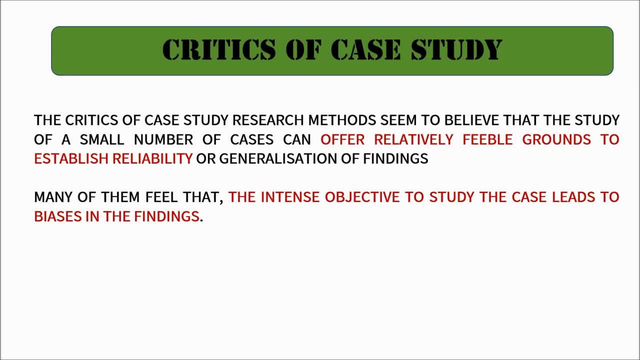 feel that intense objective to study the case leads to biases in finding what happens. we are so critical of case studies that we want to prove everything that this is the way it is happening. so many at times, in the contextual studies of cases, biasness also comes out due to the researchers. 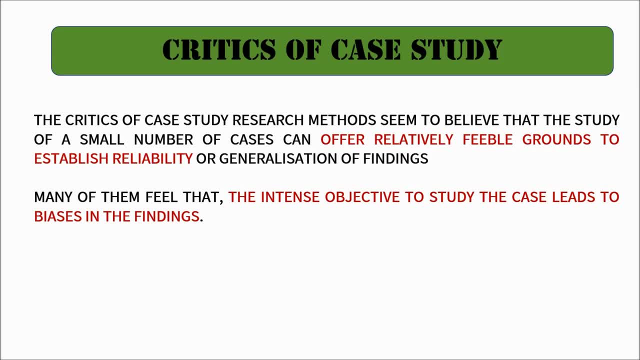 inability to understand that it cannot be generalized and do not put intensive efforts necessarily to prove a point on the ground. so what happens? these biases often keep dropping right and some also feel that case study research is only stating an, you know, as an exploratory tool. it is nothing more than an exploration tool. go to the field. 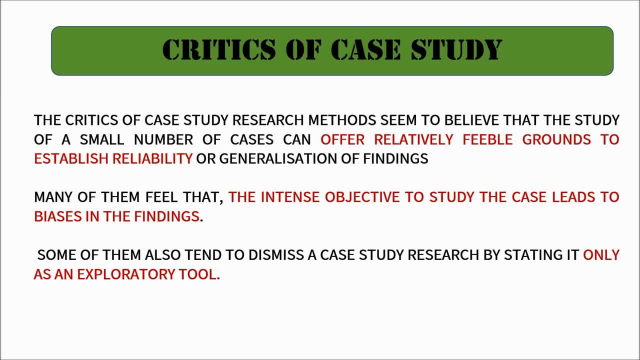 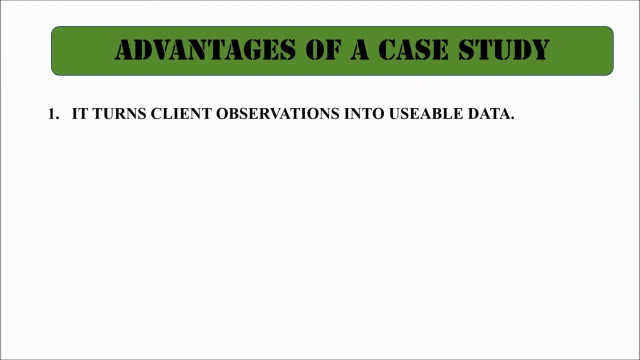 explore, ask some questions, prepare, report and come back. so it is very feeble. it has been understood as a feeble tool, just an exploratory tool. so these are the major critics of the case study. all right, now let's look at the advantages of case study. all right, so advantages- it turns client observations. 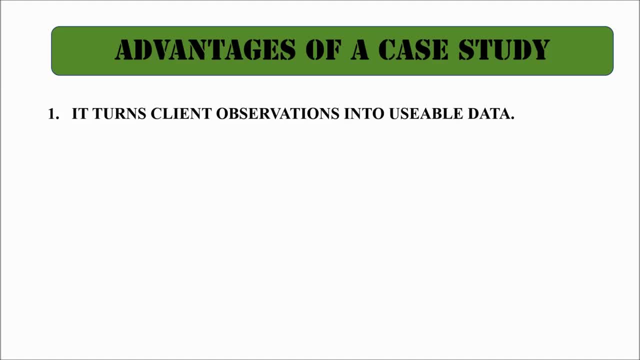 into usable data. remember, whatever is our observation is becomes a data for further research, isn't it? So it turns opinion into facts. This is very much important. It is relevant to all parties involved, whosoever is involved, whosoever are the stakeholders. 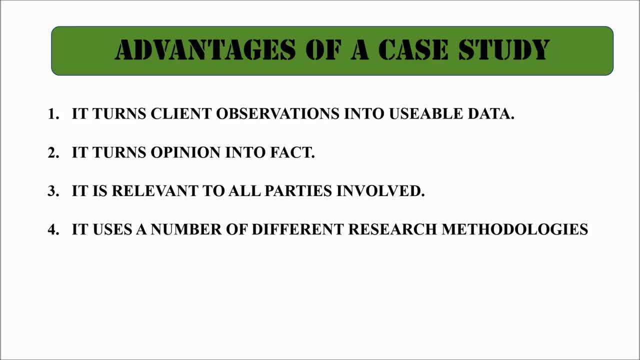 It uses a number of different research methodologies. That is the best part. It is beneficial because we can have a number of different research methodologies for case studies. It can be done remotely as well, isn't it? And then it is inexpensive. 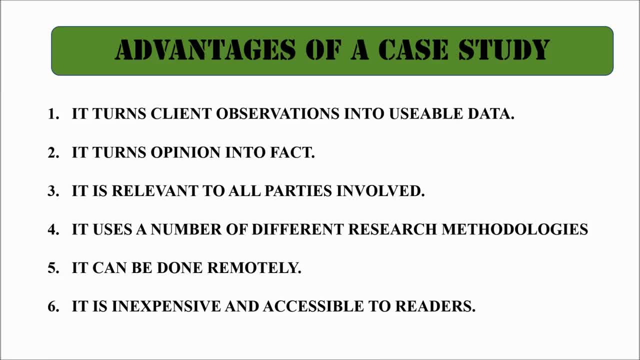 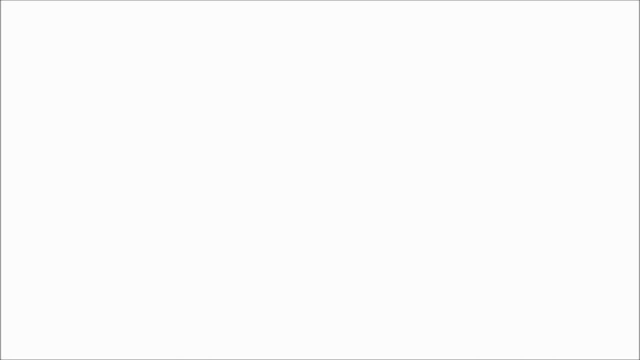 It is least expensive and that's the major feature, that it is accessible to all readers, because a report can be read by anyone. right Now let's look at the disadvantages. So the disadvantages: it can have influence of factors within the data right.